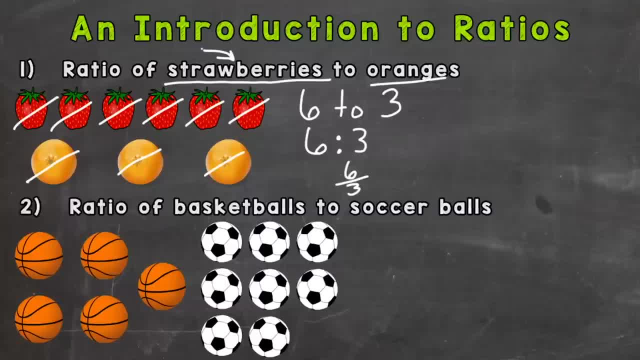 fractions. when it comes to ratios, you want to simplify the ratio if it applies, And here it does. So we need to find the greatest common factor, or what can divide into both six and three, to simplify here. And three is a common factor between: 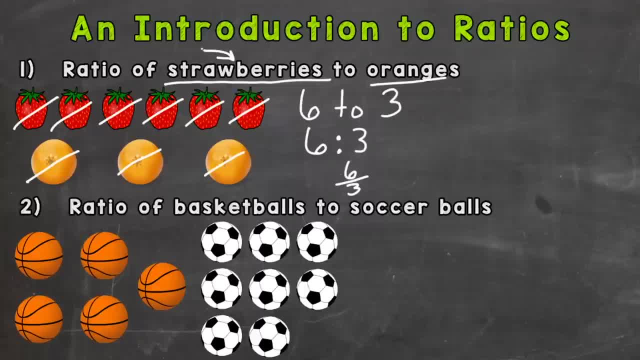 six and three, And it's the greatest common factor. So let's divide both the six and the three by three. Well, six divided by three is two, And three divided by three is one. So I'll do the colon way here first, Or I could put two to one Or the fraction two to one, And let's take a look at our. 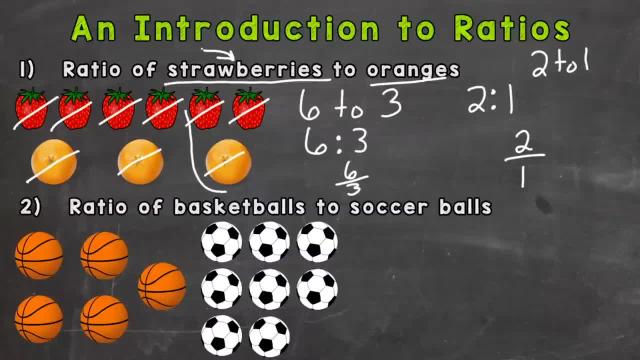 picture over here, And for every two strawberries there is one orange. so our simplified ratio matches our picture over there of the strawberries and oranges. okay, so again we can use the word to a colon or a fraction, whatever comes first in your ratio right: strawberries to oranges up here in the original. 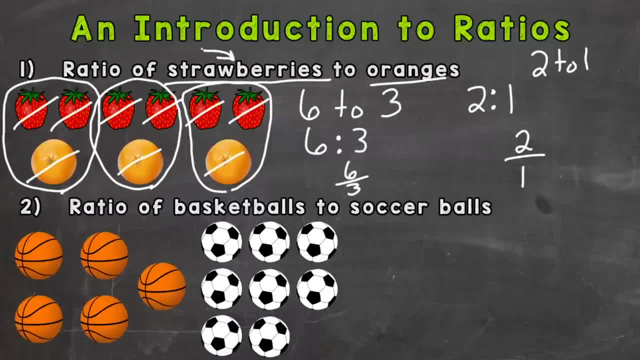 problem needs to come first in your ratios. when you write out the answer now- oranges- there could be a problem. that's a ratio of oranges to strawberries. in that case you need to put the oranges first and the strawberries second. so let's take a look at number two: ratio of 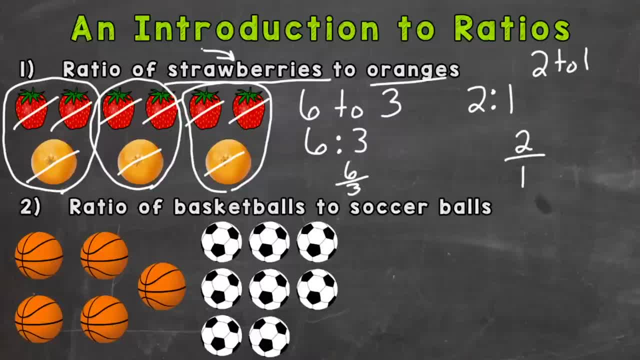 basketballs to soccer balls. well, there are five basketballs and there are eight soccer balls, so we could put five to eight, we could use a colon, and that represents five to eight, or we could use a fraction: five to eight. now, this particular ratio cannot be simplified. the greatest common factor: 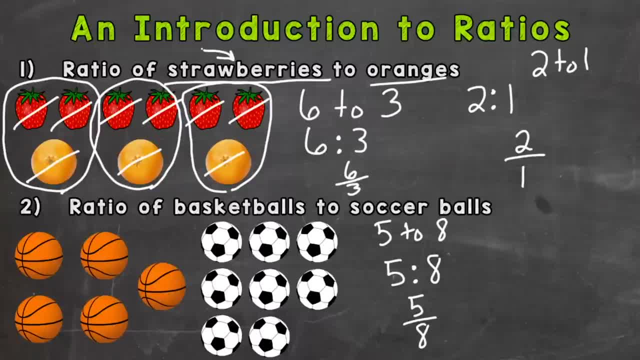 and only factor between five and eight is one, so this is simplified. so for every five basketballs, there are eight soccer balls. and remember, basketballs needed to come first because it came first in our original problem. so there you have it. there's our introduction to ratios. we learned about what a ratio is and